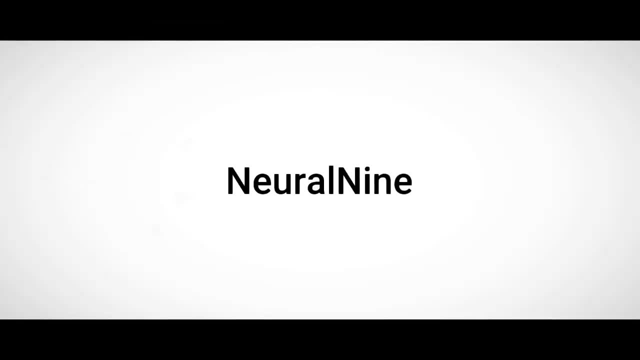 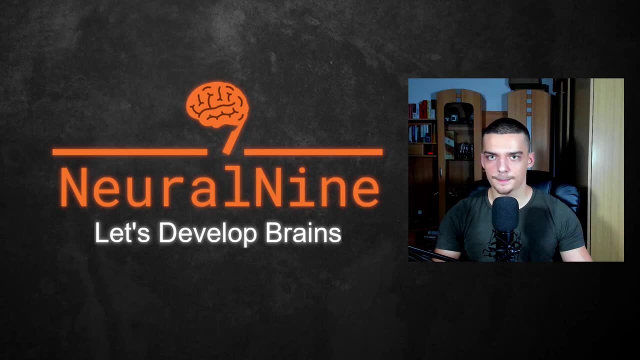 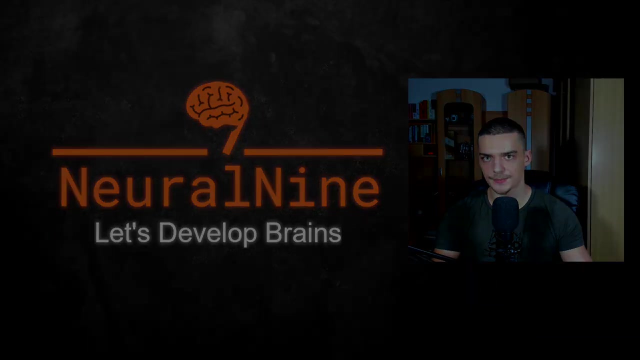 What is going on, guys? welcome back In this second episode of the C programming tutorial for beginners. we're going to talk about data types and variables, So let us get right into it. So we're going to start by defining the basic structure of the code, again like we learned in 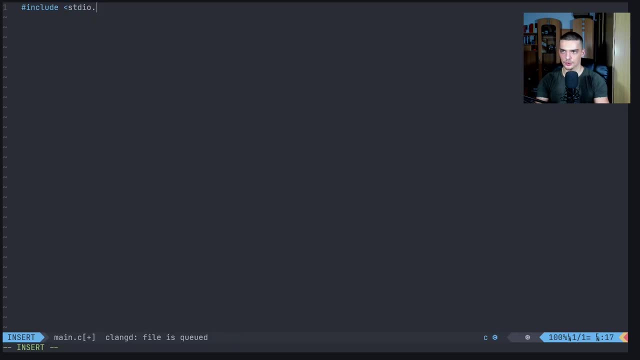 the last video, we're going to include stdio, which is for standard input output, header file, And we're going to define a main function, the entry point of the program, and we're going to again return zero. Now we're going to talk about variables and data types today, And a variable is: 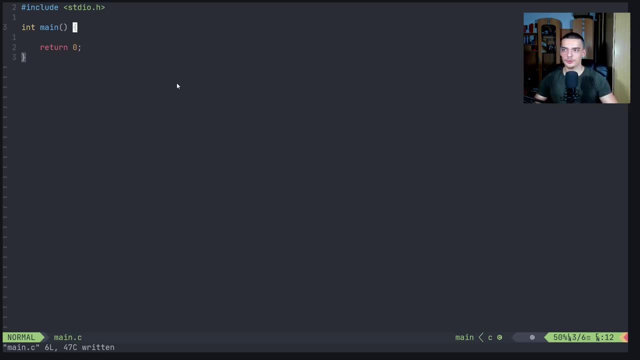 essentially just a placeholder for a value. Now, if you are already familiar with Python, for example, in Python we have variables, but we don't have to specify the data type. So in Python, what I can do is I can just say a equals 10,, for example, And that's it. I have now an integer. 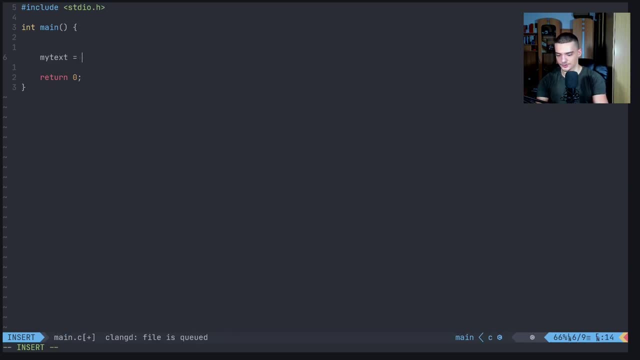 or I can say: I don't know. my text equals hello world and that's it. So I don't have to specify a data type. I don't need to do anything manually In C if I want to specify or if I want. 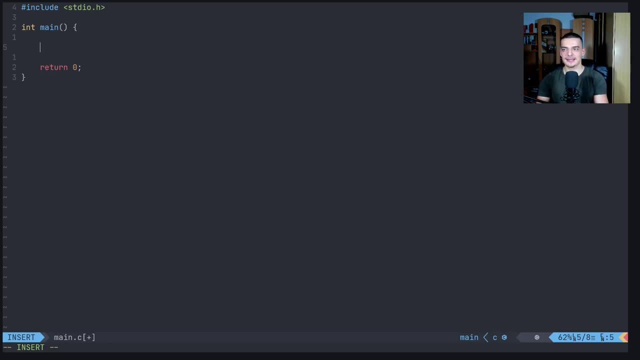 to create a variable that stores integers. I need to specify that this variable stores integers. So I need to say int a equals 10, for example. or I can also just say int B without assigning a value. So this would mean that B is essentially just defined but not assigned. So 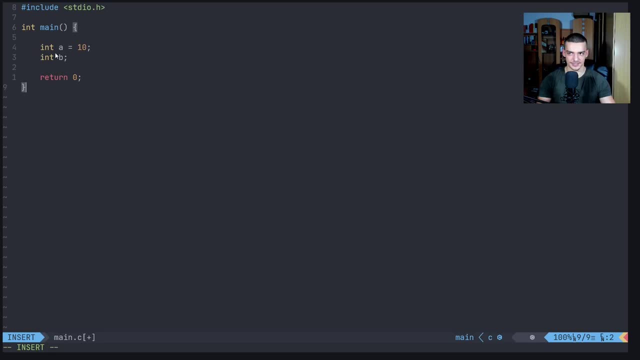 B is whatever it is, but it's not. it doesn't have a specific value assigned, And this is how you do it essentially in C, and we have different data types with different sizes and with different minimums and maximums and so on. So this is what we're going to talk about in today's. 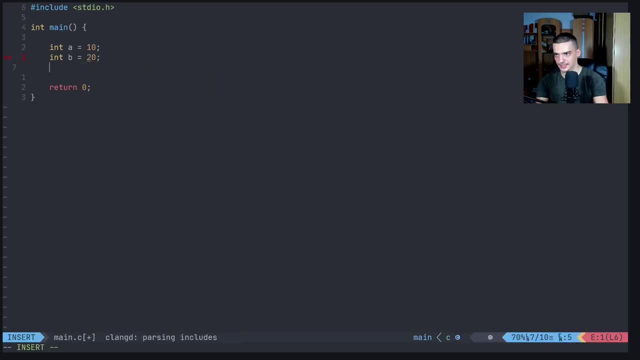 video what we can do here right away, so we can say: B equals 20.. And then we can go ahead, for example, and say: in C equals A plus B. And now, whenever I use C or A or B, this refers to. 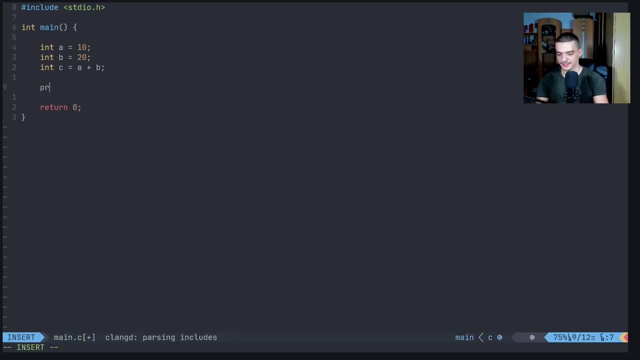 the value B Behind that variable. So if I go ahead and say sorry, if I go ahead and say print F, and then percent D plus percent D equals percent D. Remember, this is the placeholder that we learned about in the last video. then a backslash in here for the new line in the end, and I pass A, B and 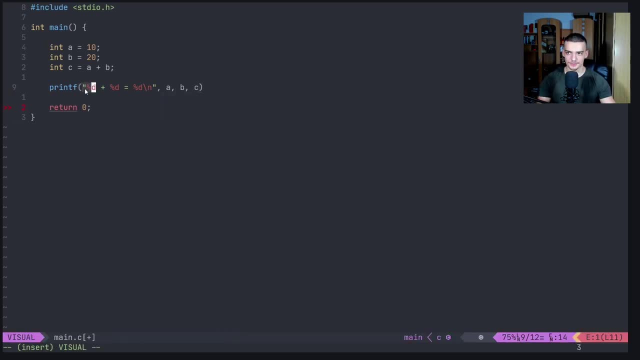 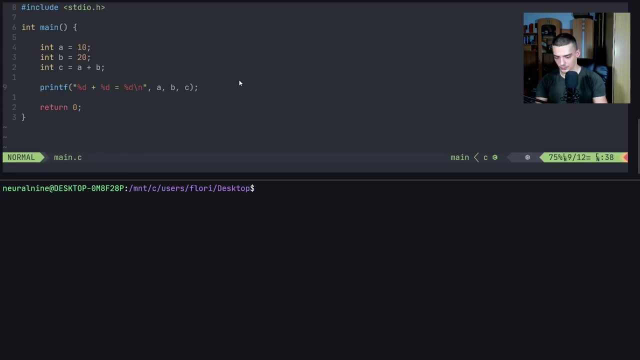 C. What happens is that the first placeholder is filled with a, the second one is filled with B, the third one with C, and the result is obviously 10 plus 20 equals 30. So let me open a terminal down here And let's go to. we are already at the. 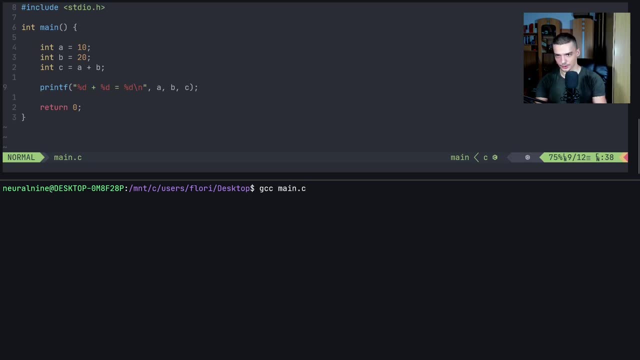 desktop. So GCC, again main dot C. So we're compiling, the output is going to be main And in order to run this now, point slash main And you can see: 10 plus 20 equals 30.. This is what we. 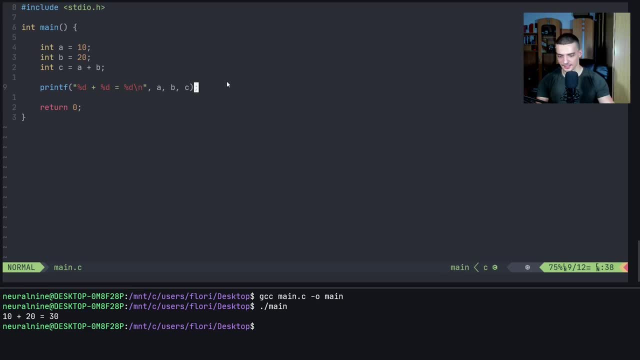 printed. So this is very basic. I think we can also. I'm not sure if this is possible, but I think we should also be able to do it like that. Let's see, Maybe not, maybe yes. So let's gives me a warning. Okay, sec fault, So we need to use a. 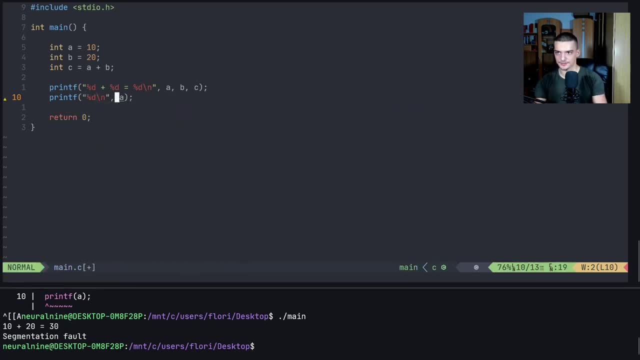 placeholder we need to say percent D backslash n, like that we can just print the individual numbers as well. But we can use now these variables And of course they can change the value. So I can go down here and say: A equals 30. Now, and then the results are going to be: 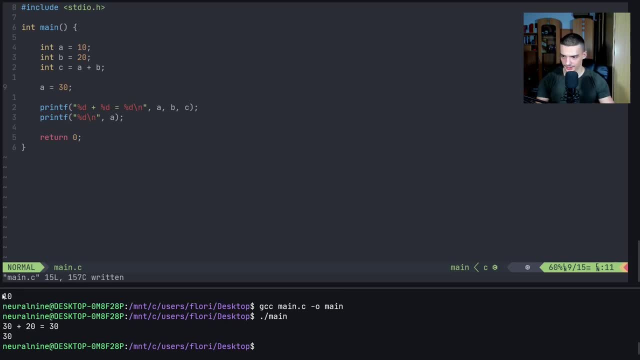 quite different. There you go, So you can see: 30 plus 20 is 30. But this is of course not right, because C was calculated when A was 10.. So I can also take this line and put it down here, And then we're going to. 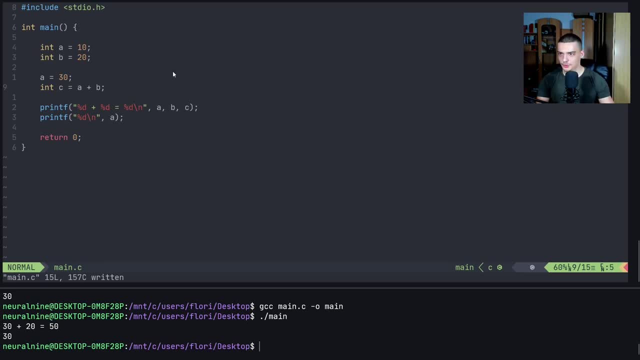 get the proper result. However, we're not going to talk about calculations here. what I want to talk about is the data type integer, And it's important to understand that different data types have different sizes. For example, the integer is defined to have at least two bytes. Now why at? 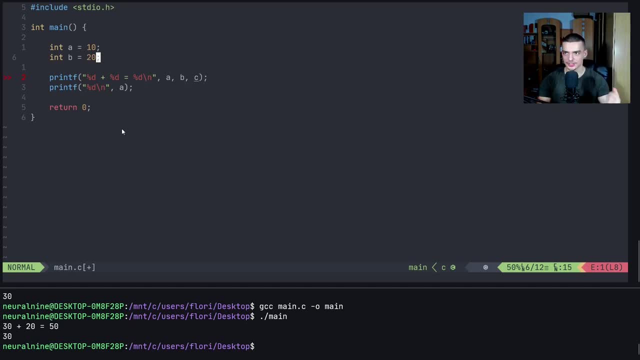 least because in C we're going to have at least two bytes. Now, why at least? because in C we're going to have at least two bytes. Now why at least? because in C and we're going to have this pattern, a lot, a lot of things are undefined. The size of an integer is undefined, I mean. 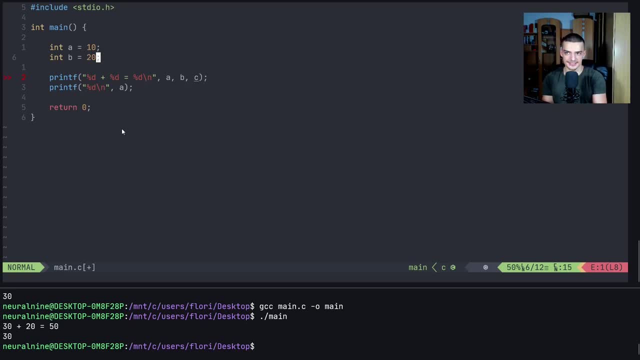 not completely undefined, but it depends on the operating system. we know that it has to be at minimum two bytes, And I think that it's even defined as not two bytes but two times whatever. a char is a character. This is another data type that we're going to talk about, And usually a 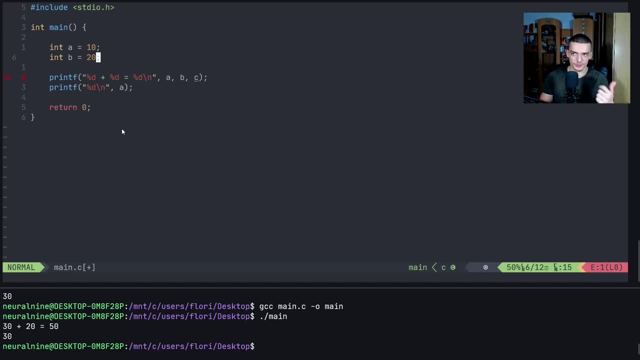 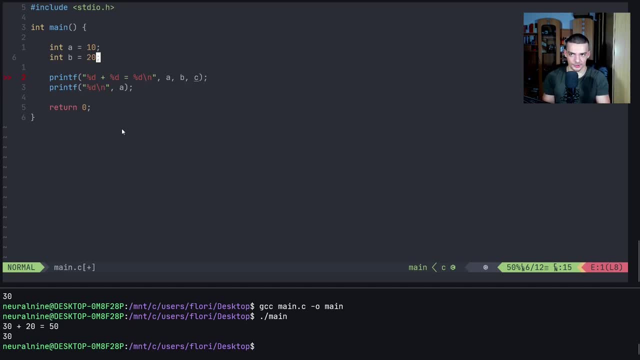 But essentially it can also be eight, doesn't matter. So depending on the operating system you're going to have different results. we can see what size an integer has by just printing it, So we can say print f And then we can use here to placeholder again, and we want to have here is: 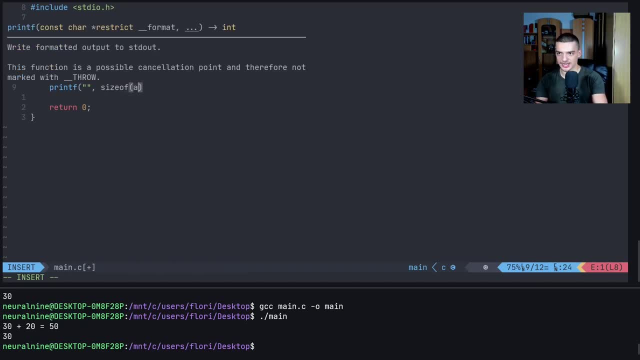 one to have size off. this is a function. we can call size off a, for example, and this is going to give us the size of the variable a, so the size of the integer a, And, if we want to format it into, 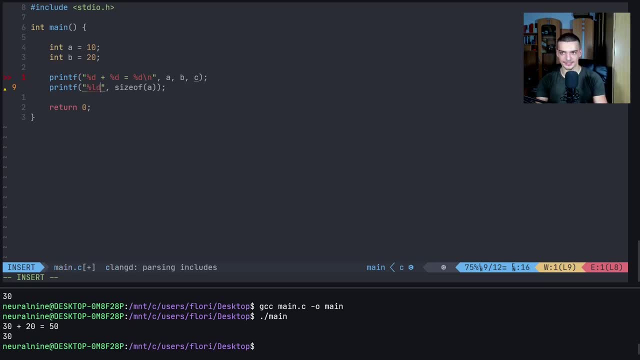 our output. we need to this time use LD, not D. why do we need to use LD? because the result of size off is actually a long integer. we're going to talk about longs in a second. here I need to define C because I undefined it. So, as you can see, now here I get four. this means that in our 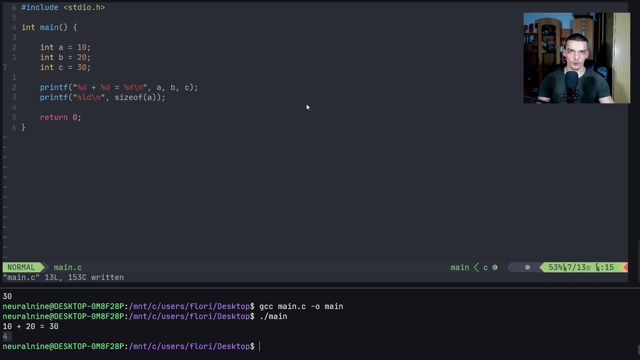 case the integer has four bytes, or four times what a character has, and a character, in this case, has one byte on my system. So this is the size. what we can also do is we can see: okay, how much can I store with those four bytes, because if I go ahead and say int, let's use 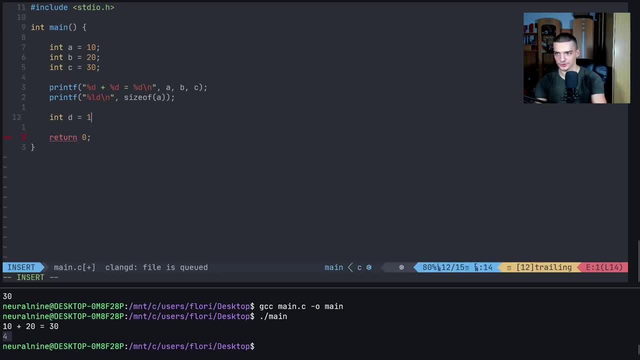 let's make another one. let's say: int D equals something like that. I think this should still be in the range. So I can just go ahead say: print f, then percent D, backslash n and then D. there should not be a problem. 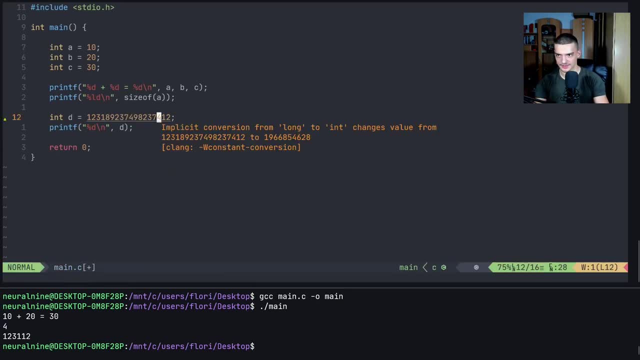 There you go, But if I go too far, if I choose something like that, first of all, you can see here that I get a warning from my checking tool here from C Lang, And you can also see when I compile. I get this warning and I can still run this, but I don't get the number that I have here. 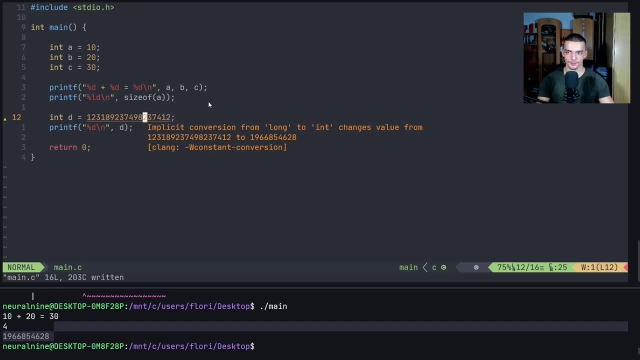 Why is that? because we have a certain maximum and a certain minimum that we can, that we can display here or that we can store in an integer, And this maximum and minimum can be seen by using a library, by including a library called. 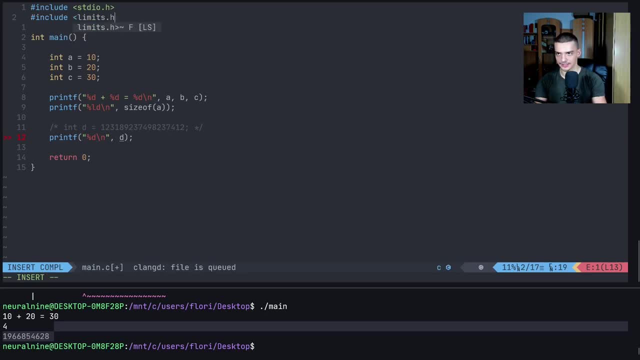 you can include the library called limits, dot h. this allows us to get the limits, And what we can do here is we can just go ahead. And we can just go ahead and say, okay, let's do this. let's say: 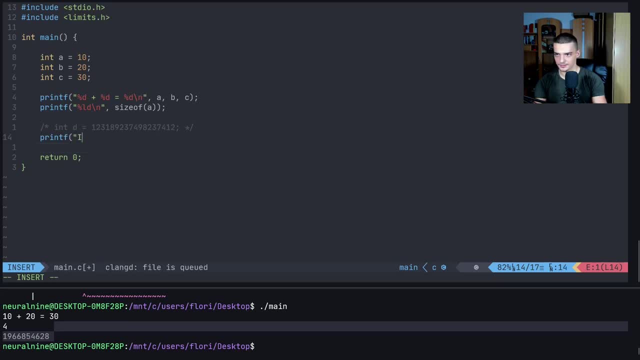 print f int max value like that, and it's going to be percent D backslash n, don't forget that. And now we can access this value: int underscore max. this is a value that we get from the limits, dot h, And I can copy this now And I can change the max to min And I can print the int min value. 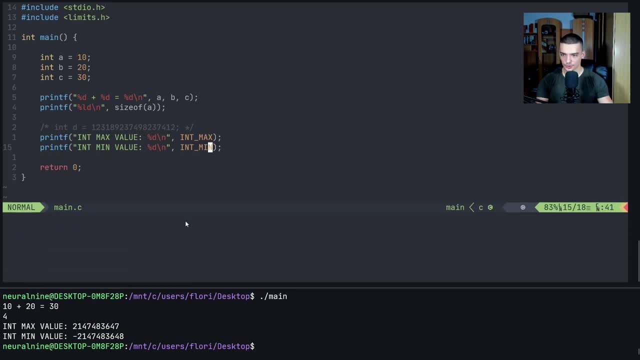 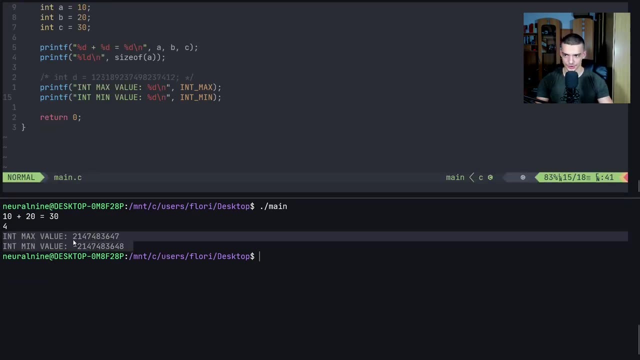 So I can compile this And now you can see what range I have When I use- let me just resize this here- what range I have when I use integers. so the max value I can store with an integer is this value. So I can go ahead now, uncommon. 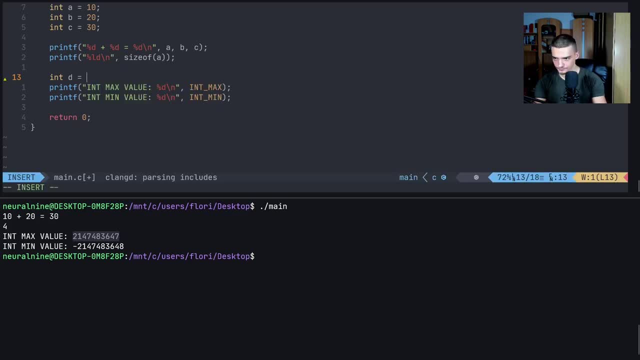 this line and I can change this value to 2147483647.. And if I now go ahead and say: print f: percent D backslash n: D, there you go. If I do it, you can see that I can display this value. But what happens if I add one more? So what? 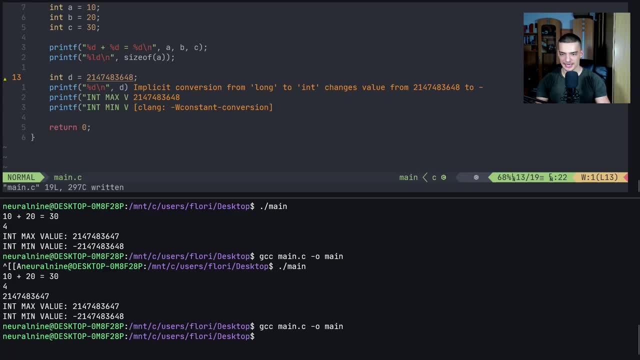 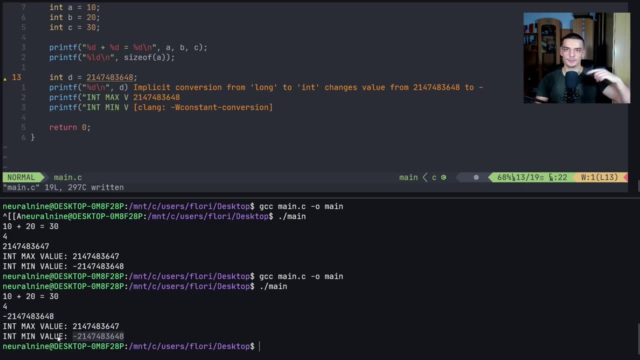 happens if I increase this by one? what you can see now. first of all, you can see I got the warning again And if I run this, you can see that I get the negative number, I get the minimum, So it basically overflows and goes full circle. So if I go beyond the maximum, it goes to the minimum. 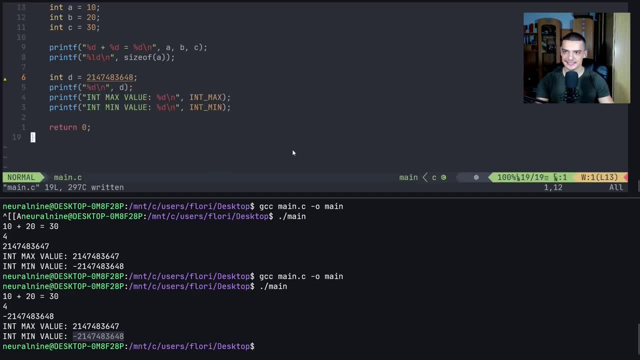 again. So that's what happens here. This is what you can store with an integer. Now, if you don't need that range because you know that you're going to have a lot of data, you can store it in a smaller number. So what you can use is you can use the short. So a short is basically an integer. 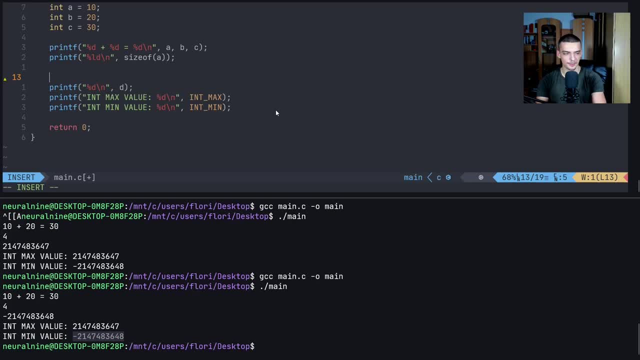 but it's less than what an integer is capable of. But again, remember, this is a minimum. So in this case you're going to see, in my system it doesn't make a difference because a short is defined to be a minimum of two bytes as well. Now, an integer is usually four bytes, a short is. 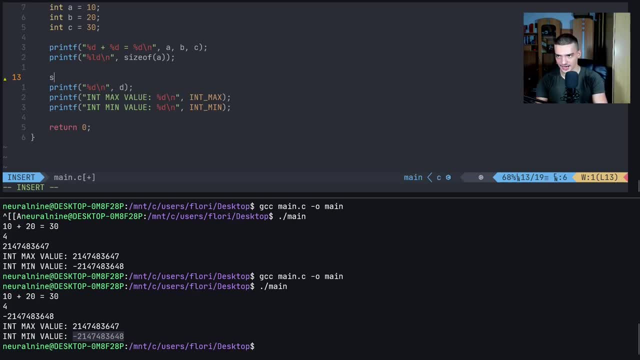 at least two bytes, and usually two bytes, But as far as I know, I think at least that on my system it's still going to have four bytes. This depends, this is undefined, this depends on your system. But if I say short s or short d equals- I don't know- 500, for example. we can go ahead and 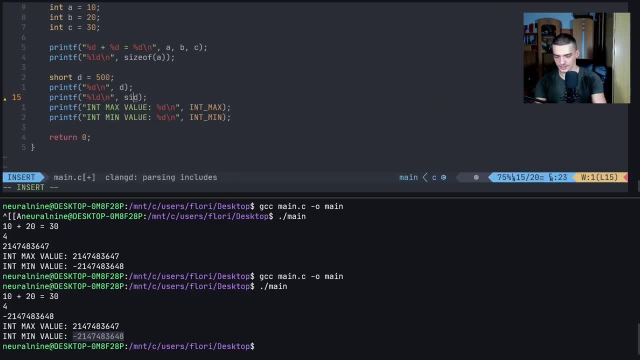 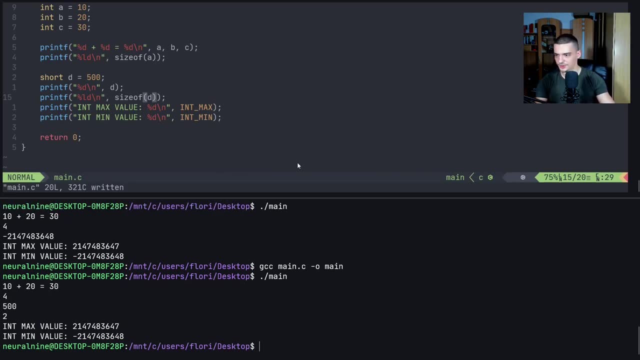 print the size of this short, So size of D in this case. I'm not gonna say it. I know what you're thinking. Oh, actually you can see that short and my system is two bytes, So I was wrong about this. 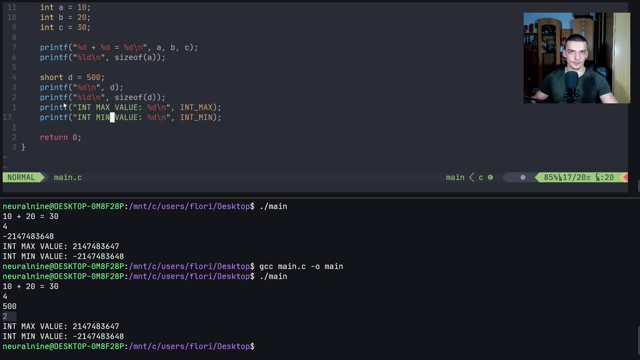 This is also what it's what is usually the case with 64 bit systems. integers usually have four bytes, even though they're defined as a minimum two byte. Even though I'm not sure I may be on a 64 bit operating system. integers have to be at least four bytes, But shorts have to be at least two. 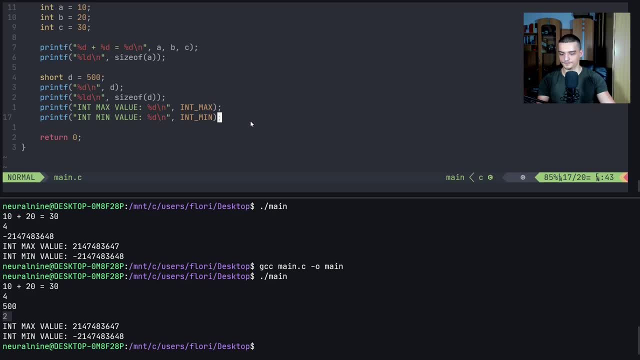 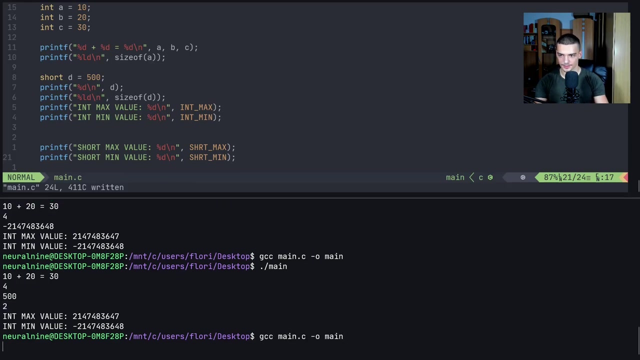 bytes, And in this case a short is two byte. If we want to see what the ranges here are, we can just copy that And we can type s h r t max and s h r t min, And here I changed this to short, short compile run. So those are the. 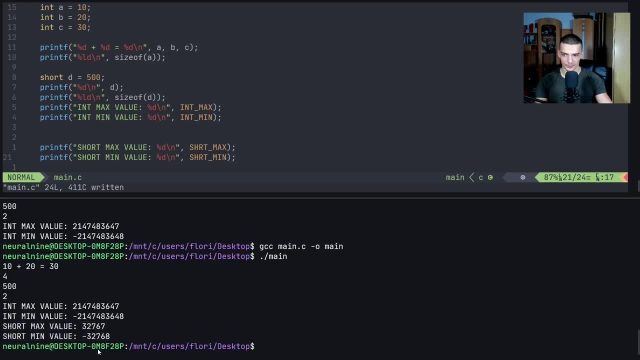 numbers. this is the range that we can use when we work with short values. Now, on the other hand, maybe you don't need less, but you need more. what you can do in this case is you can use a long, so you can just go ahead and say: 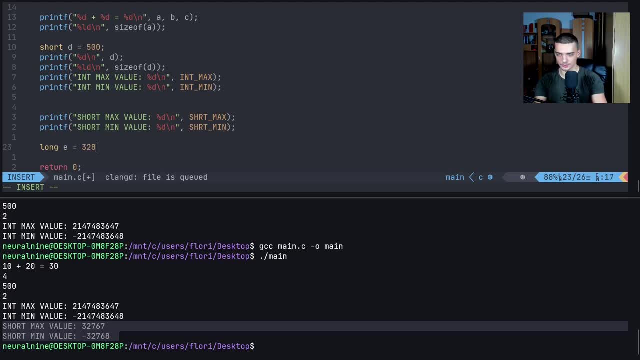 long, long, long, long long. e equals and then some large number, And then you can just print that. So you can say: print Now here you need to need to use LD, Because if you want to display a long 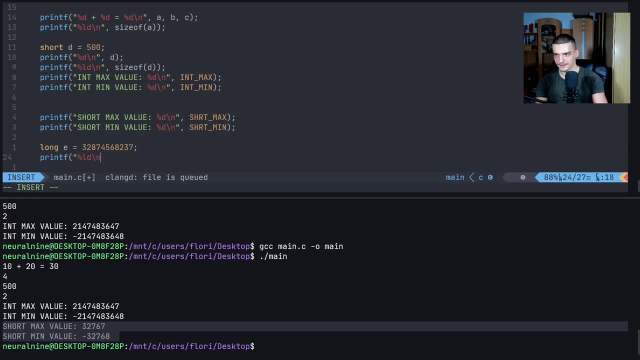 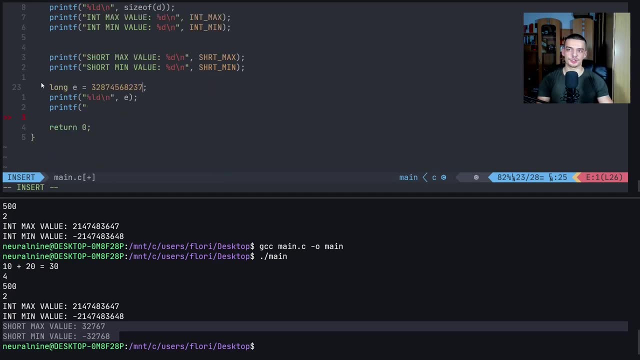 long integer. you need to specify LD, not just D, then again backslash n and in this case e, and we can also print the size. Now I can mention right away that there's not only long, but there's also long, long. So this is something that was introduced in a later standard, But you 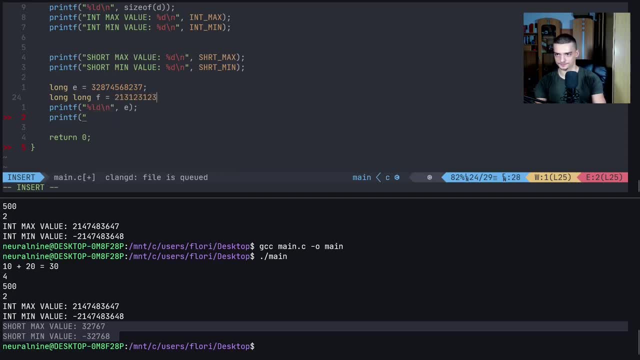 can also see long, long F, for example. Now, I think this was where I didn't have a difference. So if I now print also f and we also decide to print the sizes, so I'm going to print size long and 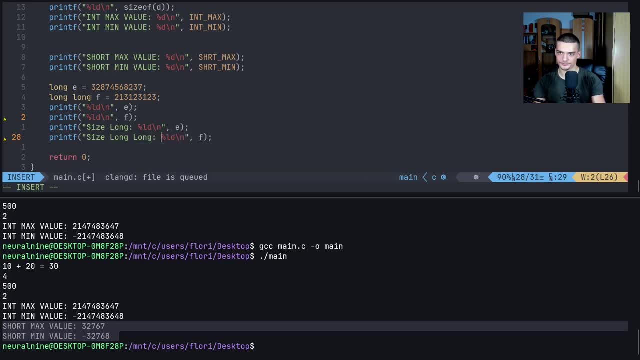 size long, long. I think that on my system I can print a size. I can also print a size for size, example, that on my system they're going to be the same. what is here? Oh, here, I think we need to add: 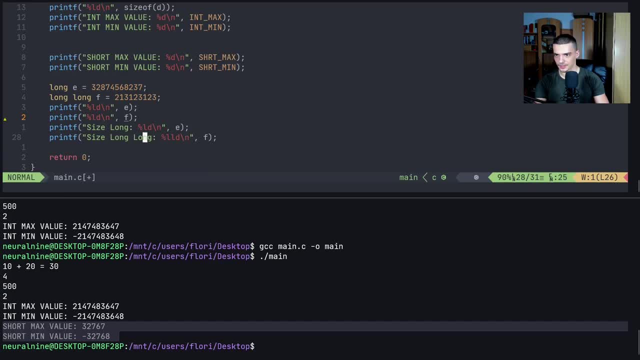 another L, Or actually for the size. not we need to add another L here. So if you want to display a long long, you need to specify LLD, And here we need to specify the size of E, size of F And I. 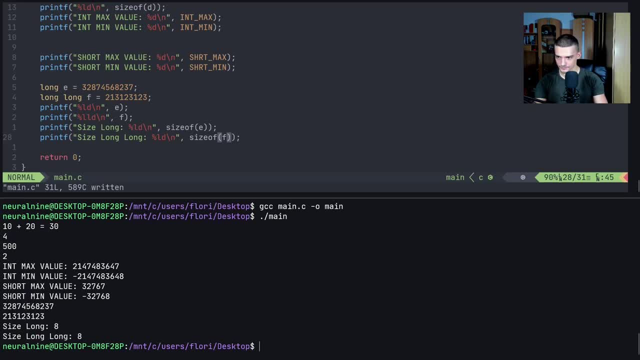 think they should be the same. here They go. they're both eight bytes. Now along, as far as I noted here, along has to have a minimum of six bytes. along, long has to have a minimum of eight bytes. In this case, along also has eight bytes. doesn't have to be the case In this case it is. 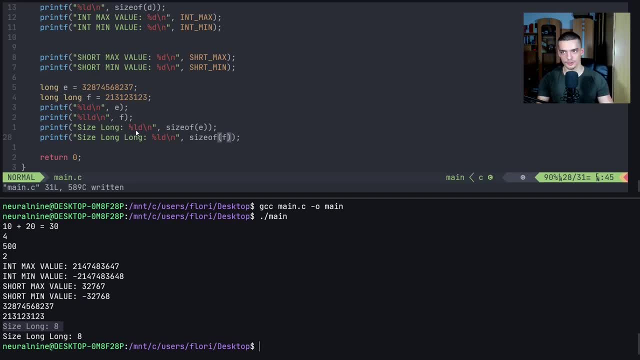 the case. So on this particular system, it wouldn't make a difference. However, if I want to compile this code for many systems, I should use a long long. And if I want to compile this code for many systems, I should use long long if I want to use the full range. Now, if you want to see the range, 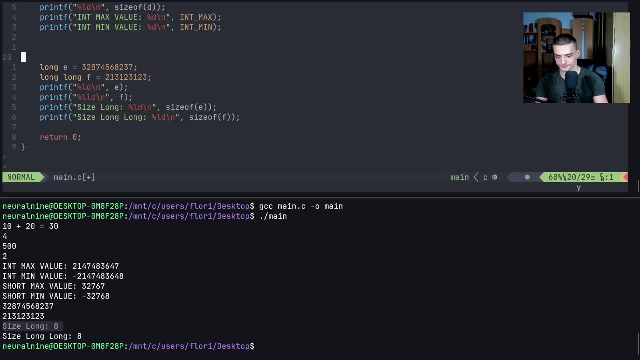 again. what we can do is we can just copy this here. Come on undo, copy this here, go down here and replace short by long, So we can. let's just look at the maximum value. So long max and long, long max, And here we're going to say long max and 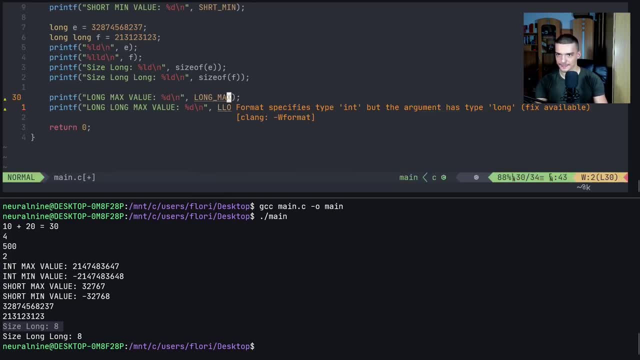 long max. And of course here we need to also specify LD And LLD. those are just placeholders. there's not really a logic behind this, is just long. I'm not sure what D stands for. I think decimal maybe, or. 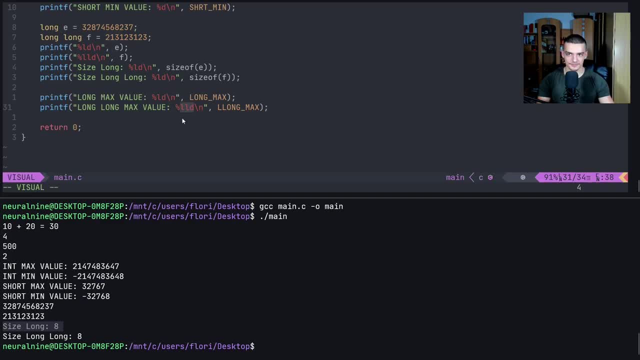 something representing a number, And LL means long, long obviously. So if I go down here and I compile this now, you can see those are the maximum values. Now, in this case it gives me the same value. Usually it's not the case, it's just the case on this particular system, usually a long has to store. 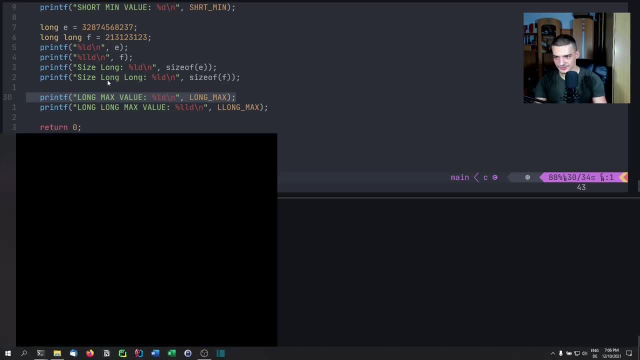 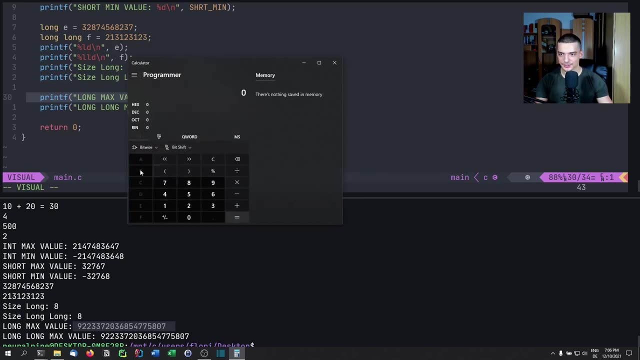 at least six bytes, so it would be less. If you want to calculate this yourself, you can also go into the calculator And on Windows for example, and you can go to programmer and you can type here into the binary. one byte is eight bits. So if you have come on, if you have something like 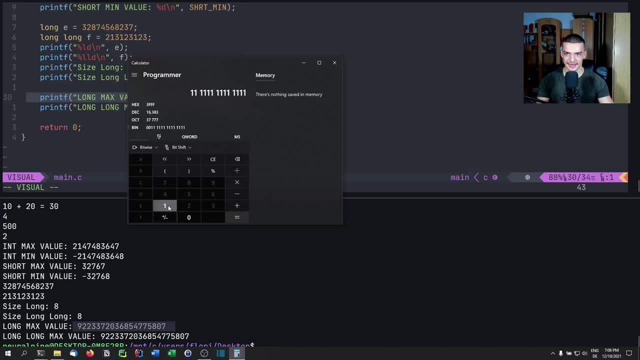 that this would be one byte And this would be two by. this would be three bytes, This would be four bytes And this is what you can store with that. So essentially you can- you can use this to find out what you can store Now maybe. 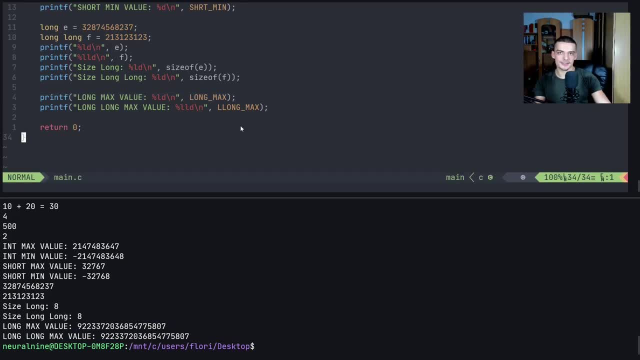 you say that you want to use four bytes, but you don't need negative numbers. So instead of going for more bytes, what you can do is you can make the variable unsigned. Now, by default, every variable is signed, So if I define Int, it's the same as saying sign, So I'm going to do that now. So I'm going to run here and I'm going to run 4 doses, Okay, so I'm going set my limit, go to the end of the program, delete copy to maximum. I'm going to go to full stop and then I'm going to worry about. 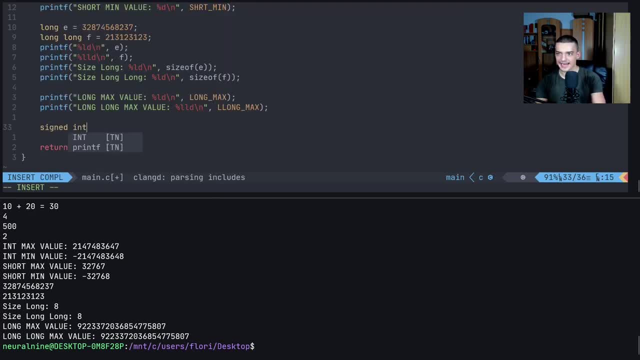 something that I don't know. I don't just know. I don't know what I'm saying. in this function, only someone. it's the same as saying signed int And what this means is that the four bytes are used for negative values and for positive values, So half of half of the bytes are used for negative values. 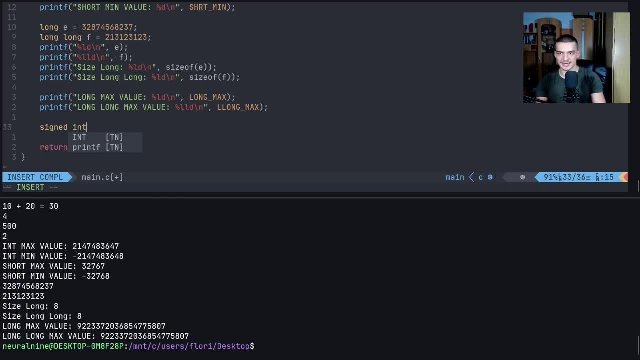 and half of the bytes are used for positive values, which means that I can store from this number up until this number. Now maybe I say I don't need negative numbers, but four bytes are enough, because I just need this and twice as much. So what I can do here is I can say unsigned int. 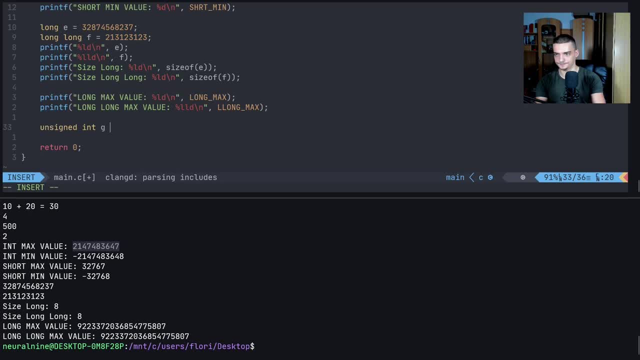 And let's call this now G. I can say unsigned int G equals, and then we can go for a number that is higher than that. So let's copy this, Let's paste this here And let's increment this a couple of times. So let's go for 9000 increments. There you go, Did this with them right now, And I 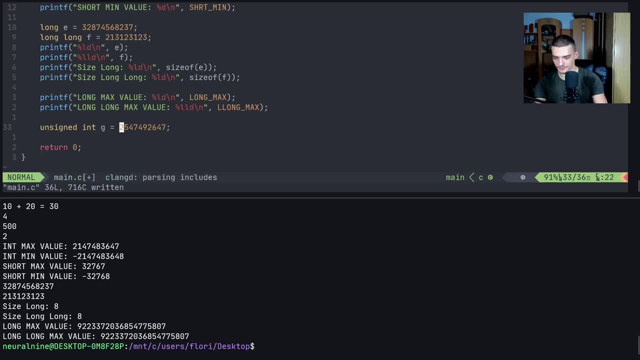 can still represent that number. I can also change this here to five, for example, and this should be three, And then I can go ahead and say: print f, D, backslash n. Now I need to say U, D for unsigned, And then G. this is important when you want to. 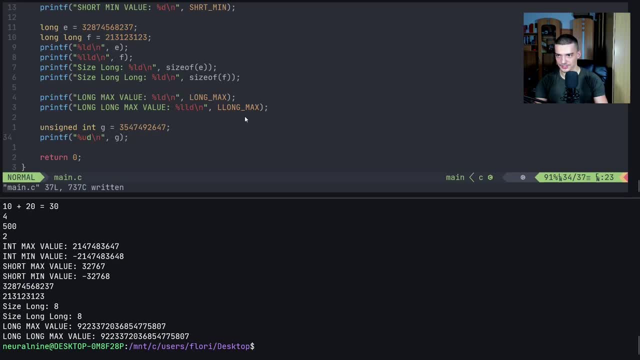 print an unsigned integer, you need to specify U D, not just D. There you go. Or actually, oh sorry, it was only U, it was not U D, it was only U have, because that is unsigned already. There you go. So now it works. Now, if you want to do the same thing with a long 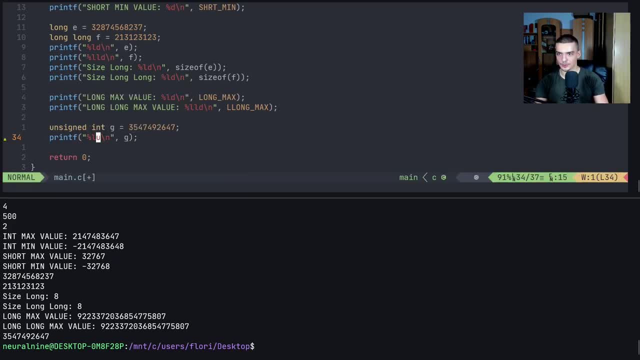 what you need to do is you need to say LU. So if you want to do this, with a long integer, by the way, saying long in and just longest the same thing. So if I want to do this like that, I can also do this. And if I want to see the limits here, all I need to do is I need to say: 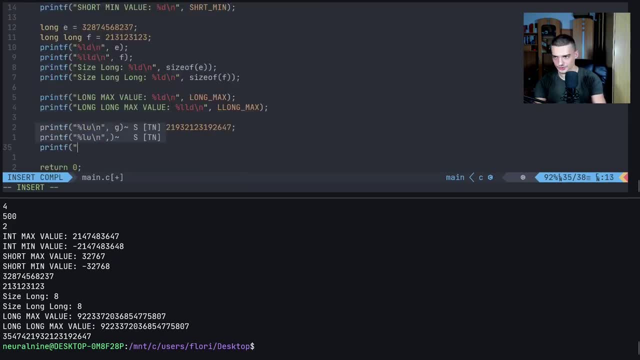 printf, And I'm just going to do this now for unsigned long, so that we don't have to go through all the examples: unsigned long, maximum, And this is going to be an ll ll you. or let's go for long, long, maximum And backslash n. What we have here is u? ll on max. this is the thing. 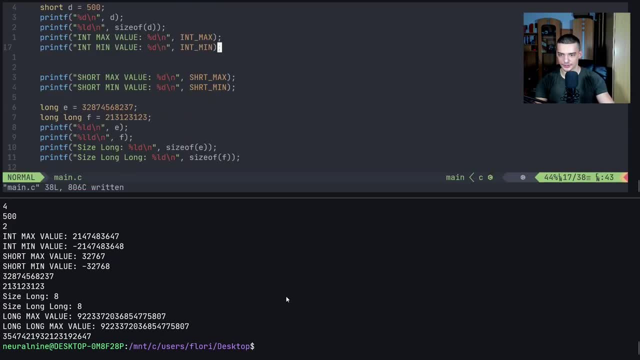 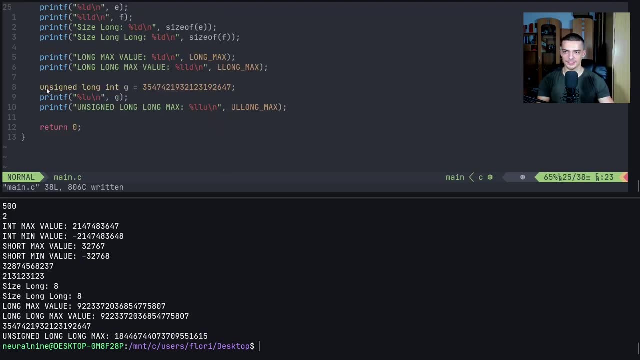 that we get from the limits library again so I can compile, I can run. this is the maximum value that we can have with an unsigned long And of course, the minimum value is zero, So we cannot go into the negatives. Alright, so let us continue. 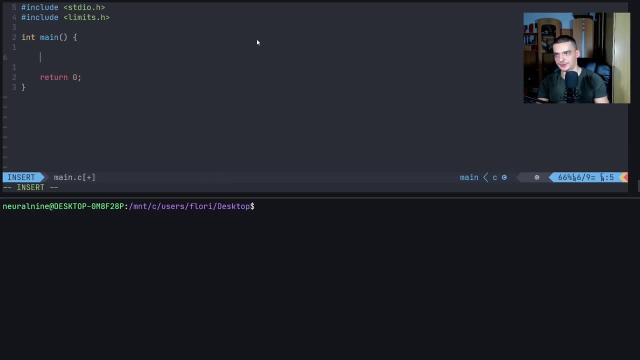 With the floating point numbers. I deleted all the code that we have up until now And what we can do here is we can specify a float variable. So the data type float is for floating point numbers f1. And this data type has a minimum of four bytes, as far as I know, and it has six decimal. 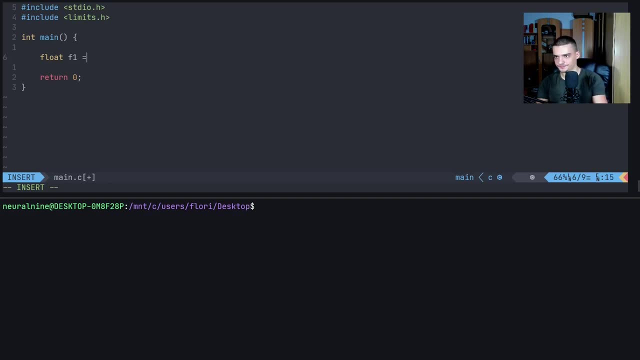 places of precision. So if I say f1 equals 12.353, four, five, six, seven, eight, nine, and continue the pattern 123456789. For example, we can write that, but the precision is limited. So first of all we can print that the 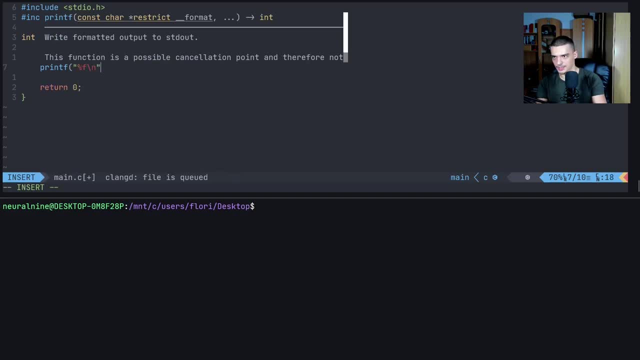 placeholder is percent f, backslash n, f1,. there you go. So there you go, There you go. You can see. first of all, it's not printed fully, But even if I specify how many places I want to print, I can. 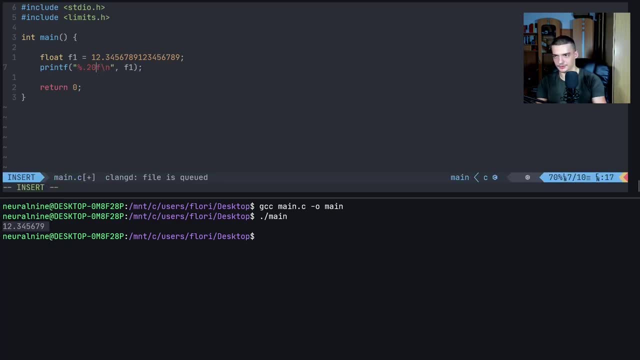 do that By saying point and then, for example, 20, to see 20 decimal places. Even if I do that, you can see that the precision is not enough: 123456.. And then it doesn't say eight, it says 9283. It's not precise. 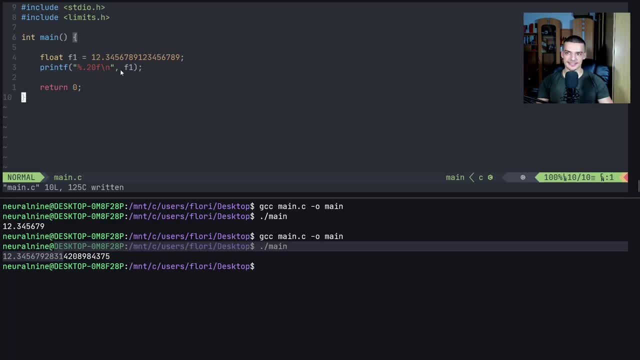 anymore. So a precision of six decimal places means that it doesn't matter where the point is. So even if I remove this here and I say I mean I don't know if it's completely irrelevant, But if I say something like that, for example: there you go, you can see that still, the pattern breaks. 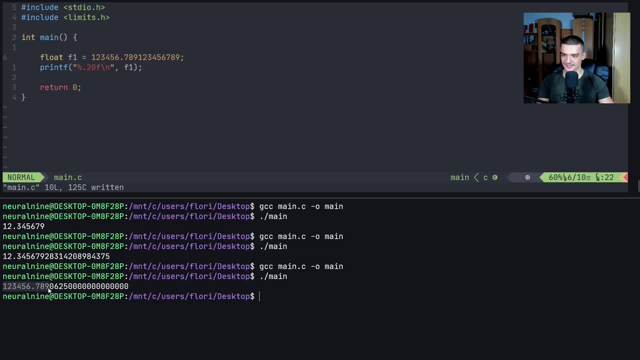 pretty soon. So we have 12345678. And then 062.. The pattern does not continue, So the precision is limited. If we want to have more precision, by the way, let me just print the size here. print f size. 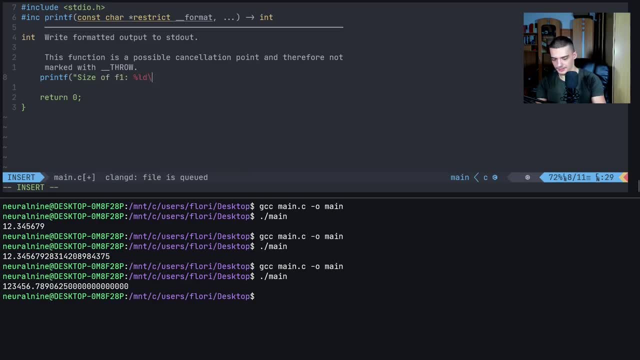 of f1 is going to be ld backslash n size of f1. And what you see here is four bytes. All right, So if you want to have additional precision, what we can do is we can use doubles. So a double has double precision. It has 15 decimal. 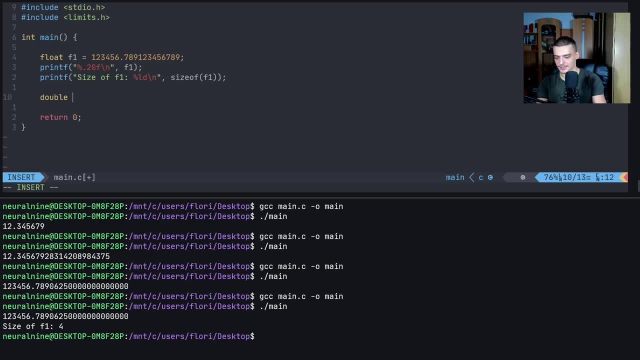 places of precision. it has eight bytes minimum. So do you want could be 123456789.. So it's the same number actually, but we're going to have a higher level of precision. so we can copy that, can paste this, we can change this to D, we can change this to D and we can change this to D. 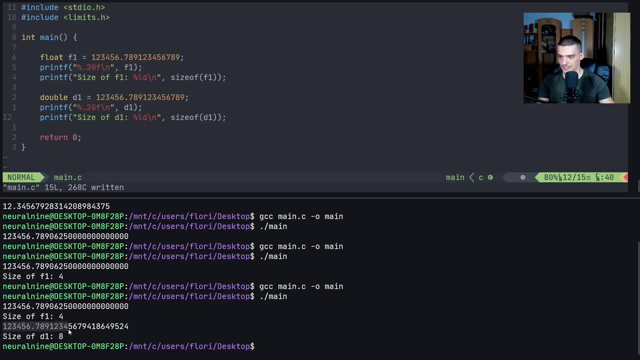 And now we can see that we have the same number, but this one has more precision for a longer time. So here we already break the pattern, here And here we continue to열. Let's on up until there. So it has more precision And it also takes twice as many bytes of space. 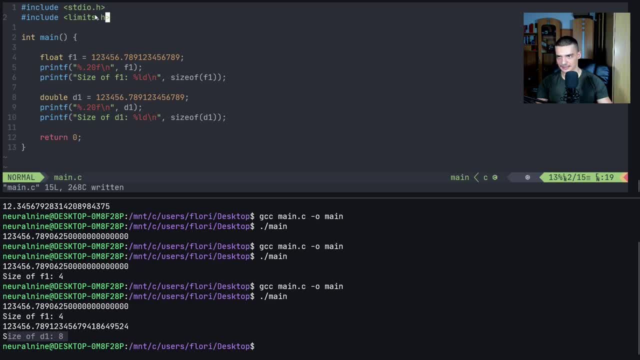 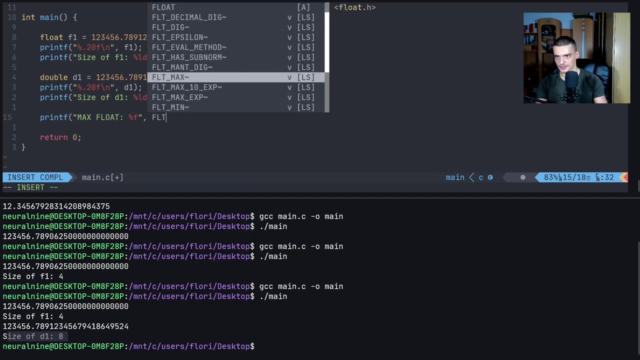 we can also take a look at the limits here. But it's not contained in the limits age, it's contained in the- I think it was- float age. there you go, And here we can then just say: print F, max, float, percent F And the max float that we can represent is fl T max, And I think we should. 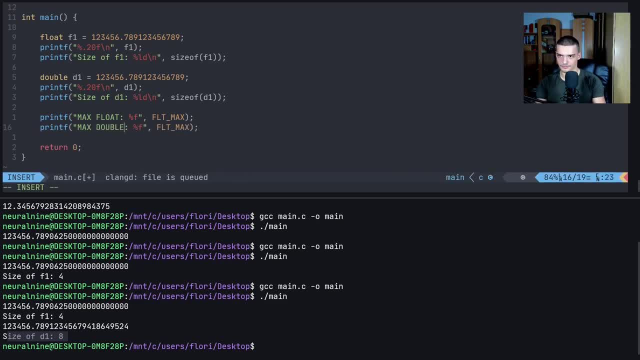 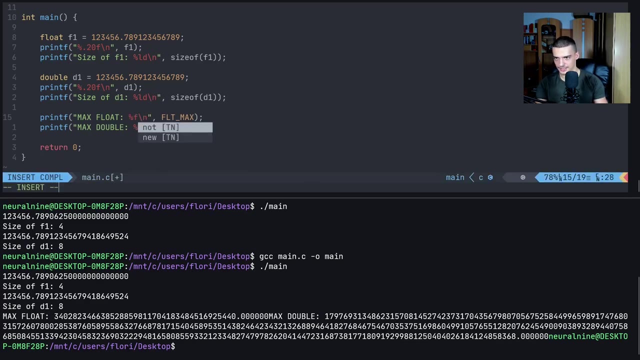 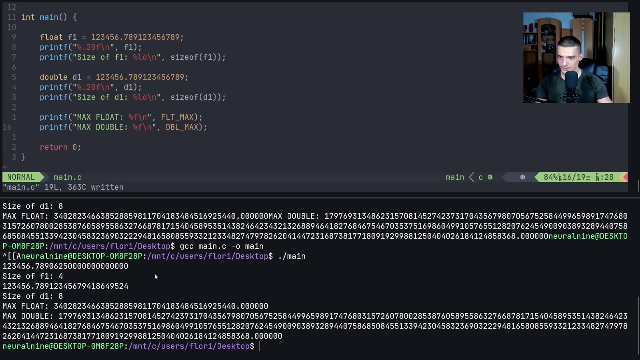 also have something for the double. I think so. at least d bl max, And we should probably probably work with backslash in here. There you go. So the max float is this and the max double that we can represent is this, But keep in mind there is a precision limit. So this is this has. 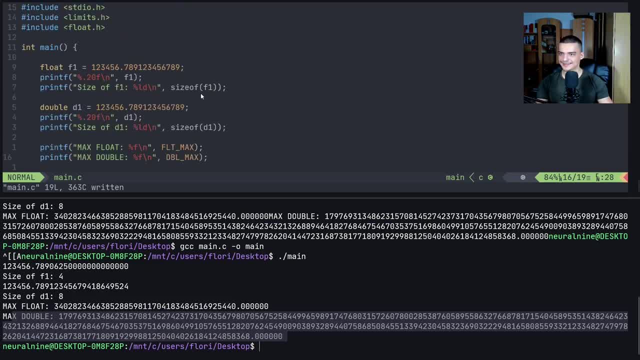 to be taken with a grain of salt. Okay, so besides that, we also have two more data types that I want to talk about in this video. everything else is going to be more complicated, But those are the primitive data types here. One is one that we already talked about, And this is the character. 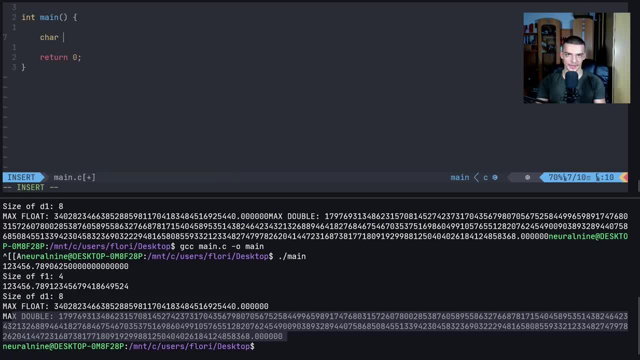 for the char, And this has usually one byte. every other size is defined in terms of the char. So an integer has to have twice as many or four times as many as a character. a short has to have twice as many as a character. a long has to have six times what a character is a long, long, eight. 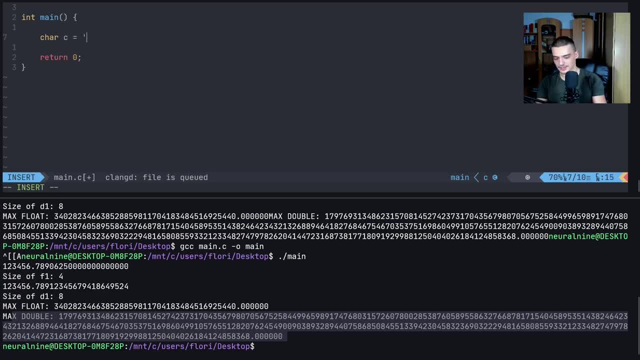 times what a character is, and so on. So the characters, see, is indicated here with single quotations- can be a, for example, a character c two- let's call this c one- can be also 30. So we can also store numbers in there, And then we can. 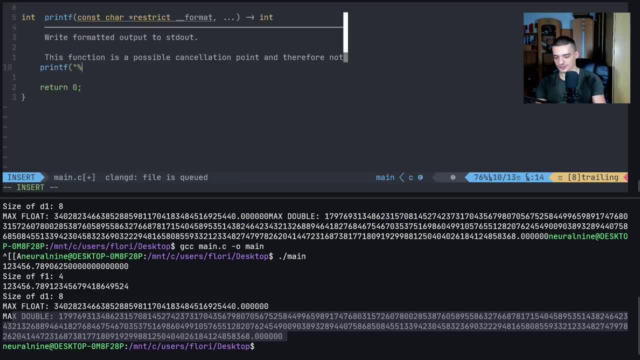 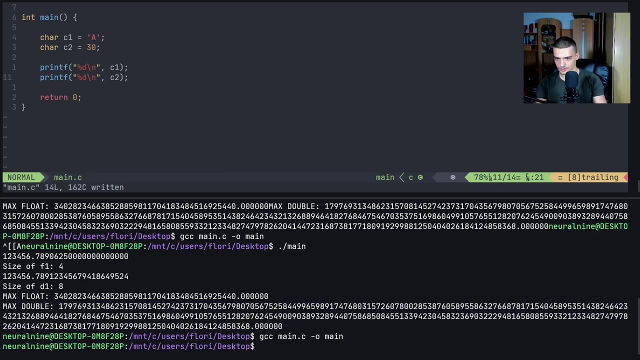 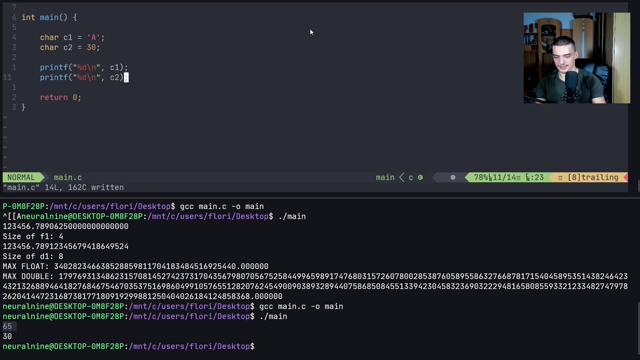 represent this in different ways. So I can say: print f, percent d if I want to represent it as a number. So I can say: percent d backslash n, c one. I can copy this and also represent c two And you can see it works. Now this is the ASCII code of a, And what I can also do is I can represent: 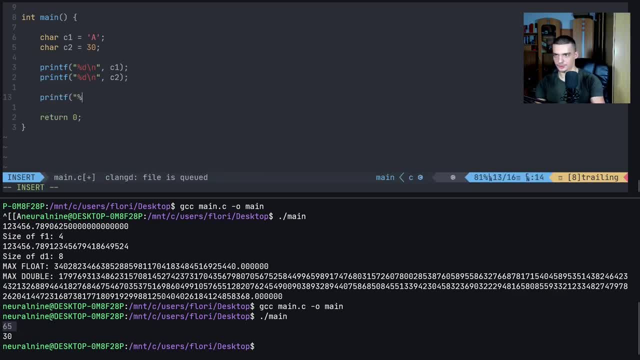 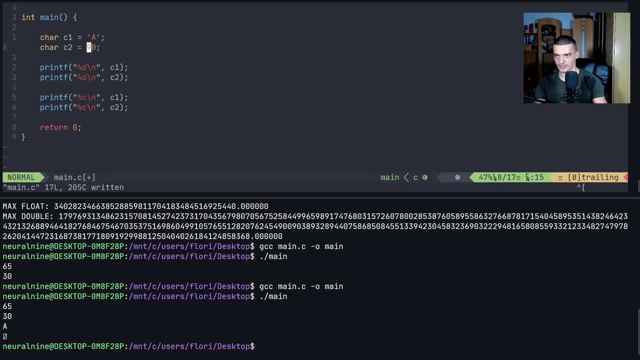 this as a character, So I can say: print f percent, c backslash n, c one, And I can do the same thing with c two, And in this case this is not a good character. Let's go with 90. Maybe, Yeah, 90 is. 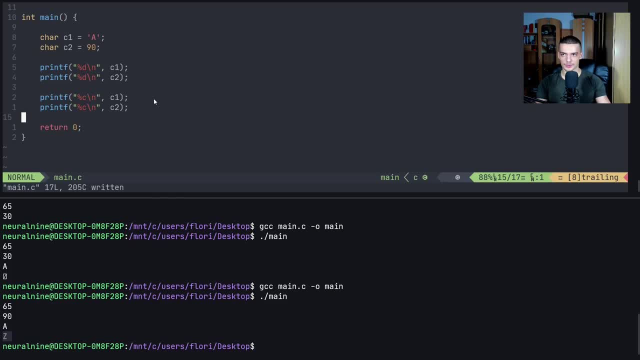 not a good character. So I can say: print f percent c. So you can see that we can work with characters like that. Now what we can do here is we can say: print f ld backslash n size of c one, for example, And you will see that it takes one byte. Now, it's not guaranteed, but it's usually. 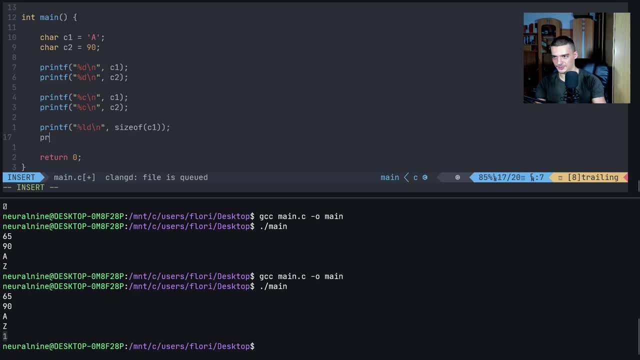 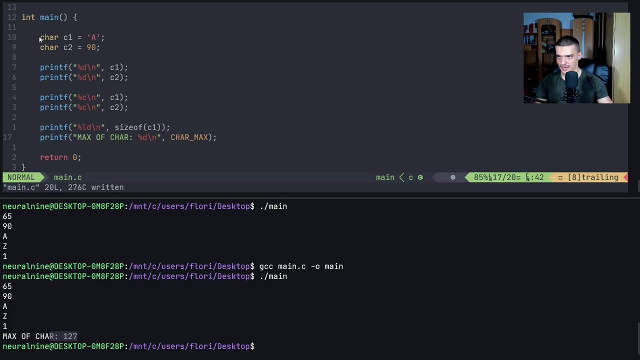 the case that a character has one byte And we can also print the limit. So we can say print f max off character and then as a number, character underscore max And this is the maximum. Now, of course we can also have an unsigned character. 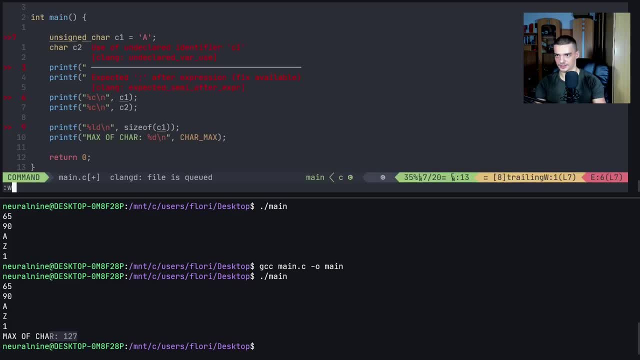 So if I say unsigned character, then probably I should change this to you. This did not work. Why didn't it work? unsigned character Max? Oh, because I'm printing the max, obviously. So actually it doesn't make sense to to make this unsigned in order to get a different. 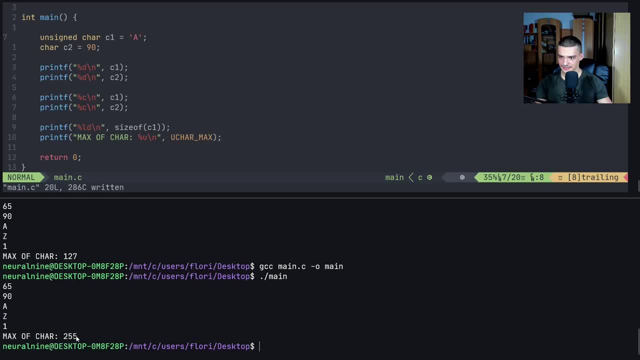 result here, But the unsigned character can represent up until 255.. And the last data type that I want to talk about is something that we know from other programming languages, But we don't have it by default in C And this is the boolean, So we can say: print f, percent, c, backslash n. 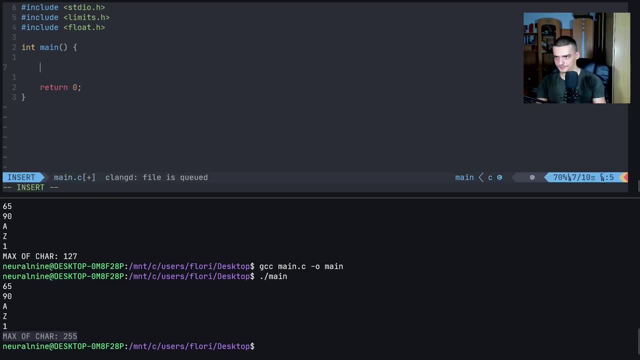 boolean. We don't have the boolean by default. If you want to use a boolean, there are many ways. we have something like underscore bool. I think this is actually available, by default even. But what I want to talk about is the std bool, So we can include here a library called std boolh. 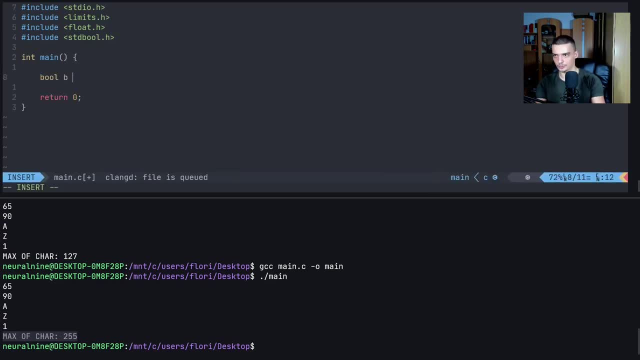 And this allows us to use a boolean. So we can say: bool b equals true, And then we can just print this, We can represent this as a number, Because that's a boolean, And then we can say: oh, fundamentally what it is, And true is going to be one And false is going to be zero. So, if I do, 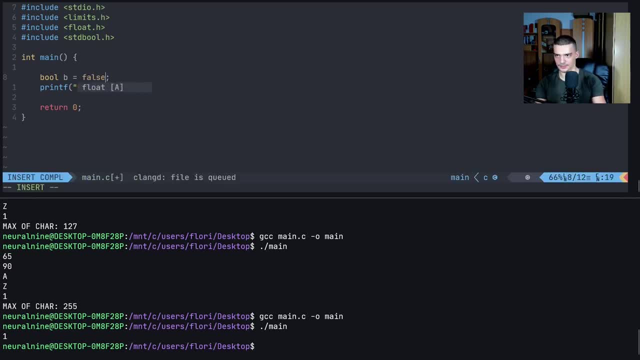 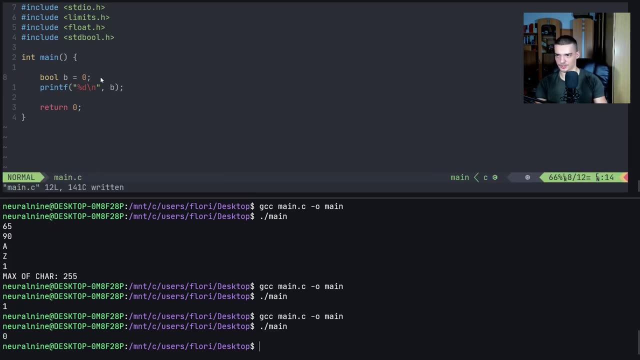 it like that, we get true, And if I do it like that, we get false. Now I think we should also be able to assign zero. I'm not sure We are. I'm not sure if we can assign a different number. 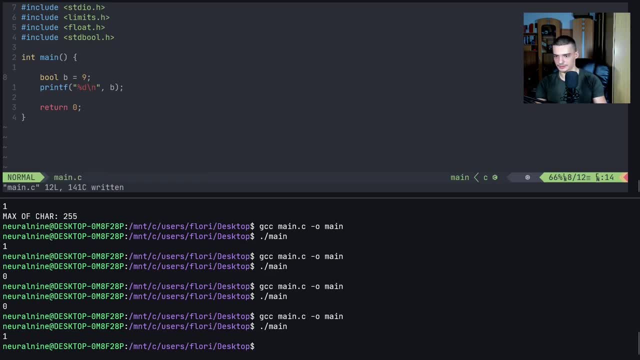 though should be possible as well. Yeah, Okay, but we still get one, because everything except for zero is one. So true, Yeah, we can also check the size here real quick, So we can say: print F and then percent LD backslash n size of B. 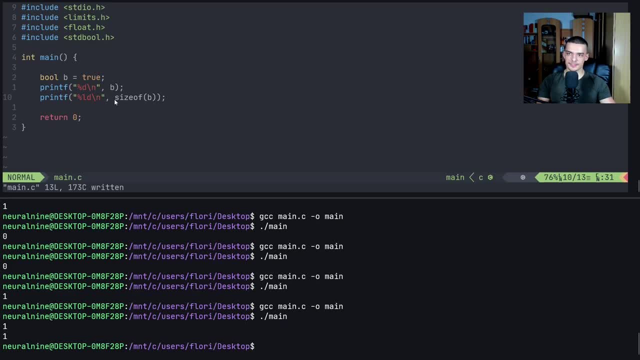 And this is also one byte, So it's important to understand that this size off basically tells us how many characters this is. So if I do this, I get one byte, And if I do this, I get one byte. So character is two bytes instead of one byte. everything has to be multiplied by two. 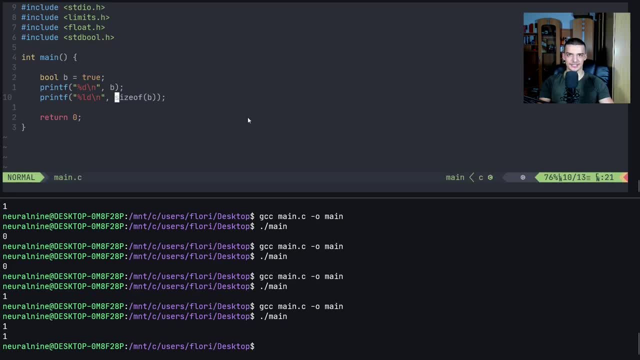 By calling size off on integer. we don't get the bytes, we get the units of characters. This is important, Yeah, So you might wonder where strings are. how do we represent strings in C? it's not that simple, because strings are essentially actually strings of characters. 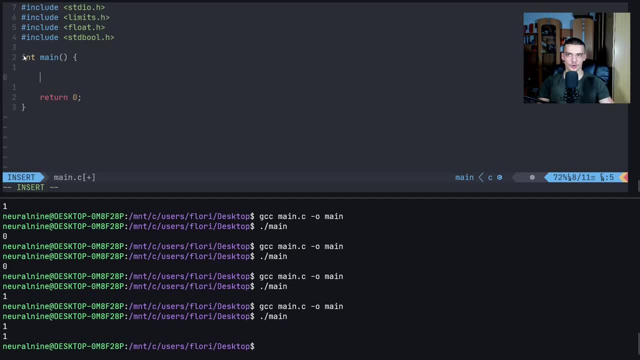 chains of characters, So this deserves a video on its own. Those are the primitive data types. we have integers, longs, short, long long. we had floats, doubles. we can also have- I forgot to mention this. we can also have. 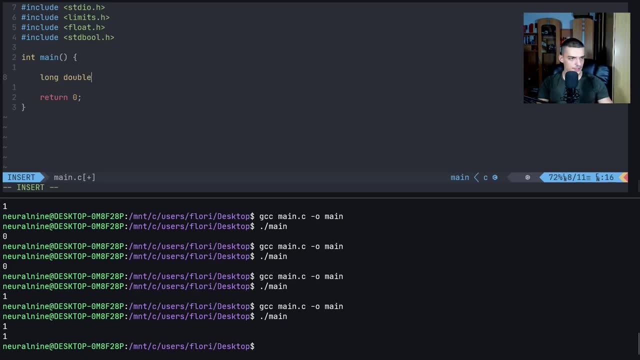 long doubles. I didn't mention that long doubles are, I think, how many bytes? with 10 bytes, I think long doubles. let's, let's try it out. LD equals whatever I want to see. if I print the size, size of LD is going to be actually LD itself. 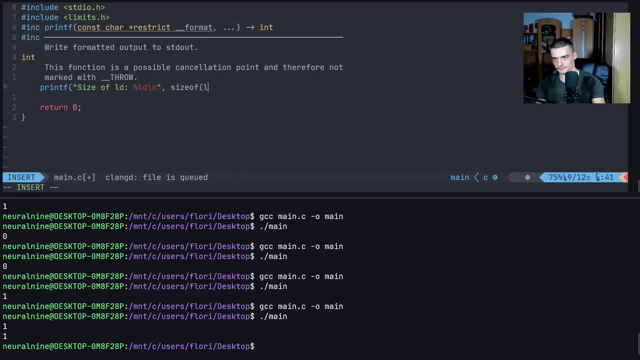 Um size of LD. Let's see what we get here. I think it should be 10.. It is 16.. Okay, we have 16 bytes. This is a pretty high precision. Okay, so we have 16 bytes when we use long double.